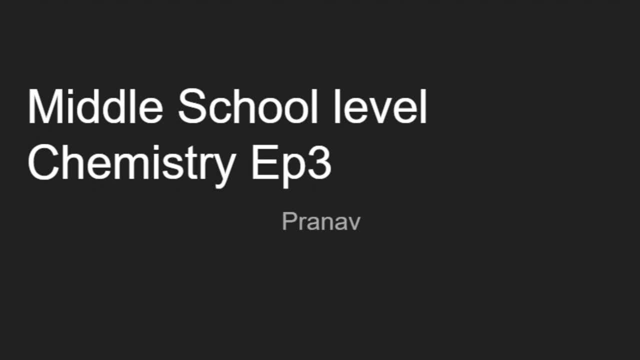 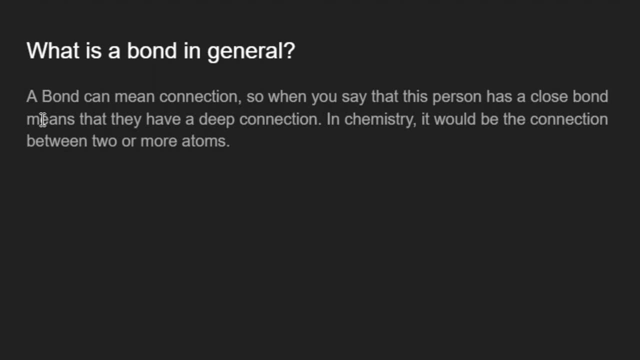 to two as the main core bonds, and we'll be discussing about that very soon, Okay. so, firstly, when we say bond, what does it mean? Okay so a bond. the synonym of a bond is like. one of the synonyms is connection. So when you say that this person has a close 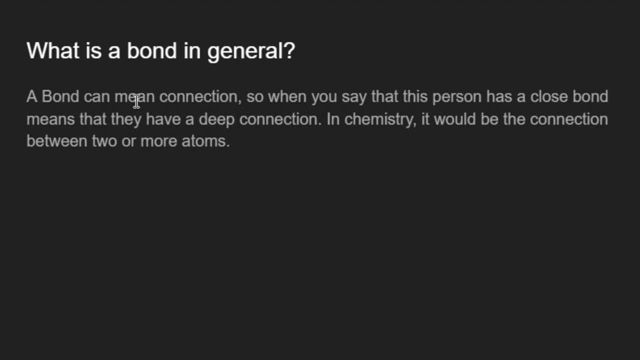 bond with this person, it means that they have some connection with each other. Now, in more chemical terms, it would mean, like the connection between two or more atoms, right And now, these core bonds that we often talk about- one of them is ionic bonds- and 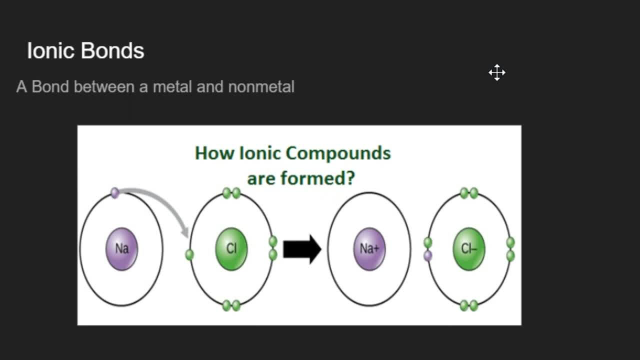 ionic bonds is basically a bond between iron and metal. Okay, this is basically a bond between metal and non-metal and not metal, And basically this bond is formed by the transfer of electrons from the metal atom to the non-metal atom. Okay, and by doing. 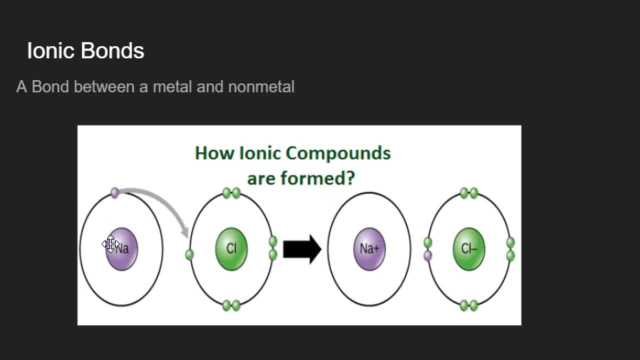 this. so what happens is that the matter like transfers, the electron, non-metal becomes positively charged, but it doesn't reach right. It doesn't reach the electron. This is when this metal loses its electron and the non-metal gains in electrons. it becomes negatively charged. 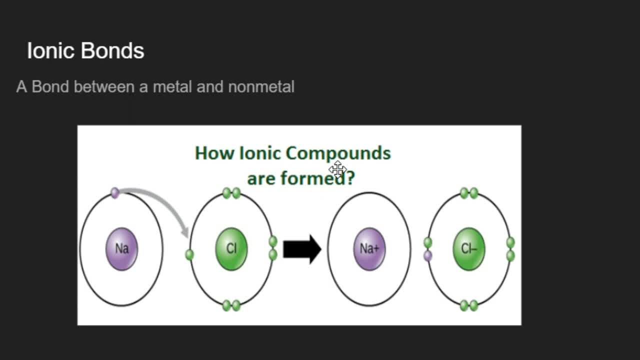 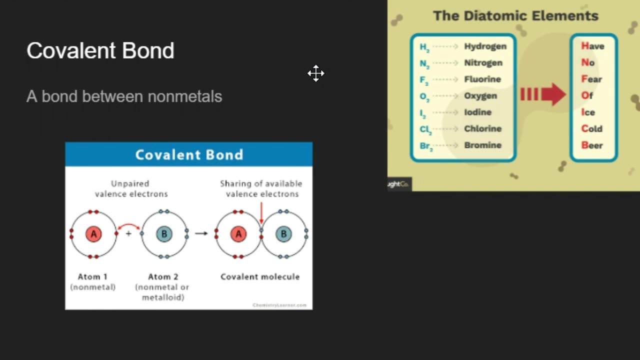 and by, and we know that, um, the positive and the negative signs are attracted to each other, and that's how the bond is formed, okay, uh, okay. the next one is called covalent bond. now, this is a another, your core bond, and this is a bond that's formed by sharing of, like valence electrons. okay, 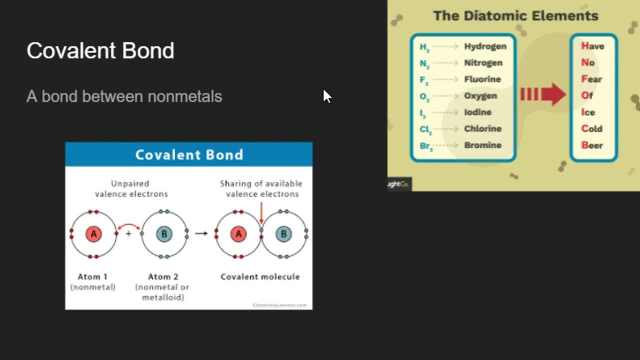 now, okay, in nature there are like some, um, some of the non-metals that don't appear as like a single atom. they're often paired right and now, um, here's like some of the lists. uh, one of them is hydrogen. hydrogen appears as h2. 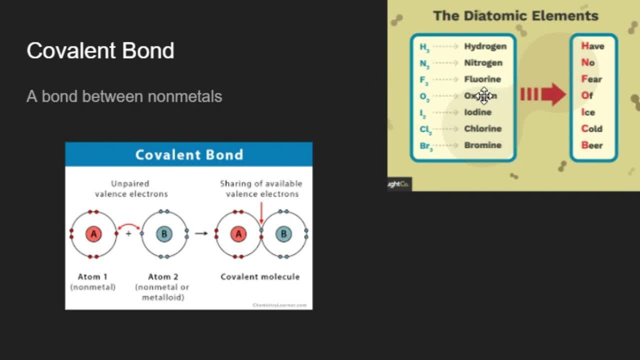 right. nitrogen is n2 and fluorine is f2. oxygen is o2, iodine is i, i, i2, chlorine as cl2, bromine as br2. now, um, keep in mind that when they're sharing the electrons, it it doesn't have to be equal. now it all depends on the atom. 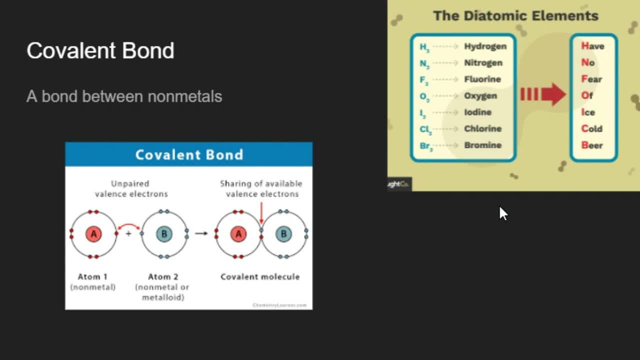 that the covalent bonds between now, if it's between, for instance, um, okay, if it's between, like oxygen and fluorine, uh, what's going to happen is the one that's more electronegative, or our electronegative basically means, like the 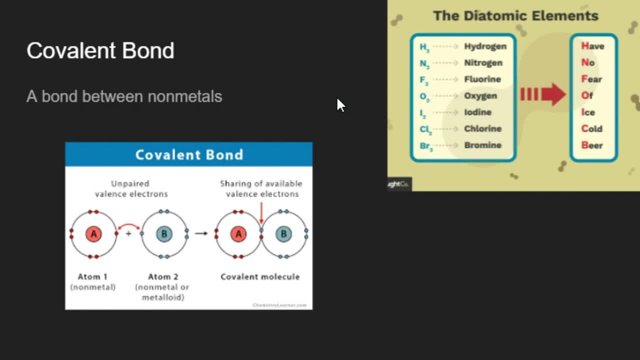 like the ability to attract electrons. okay, so if it's more electronegative, basically is that the electron would be more pulled towards it, right? so if it's between fluorine and oxygen, obviously we know that, fluorine being the like the highest electronegativity. 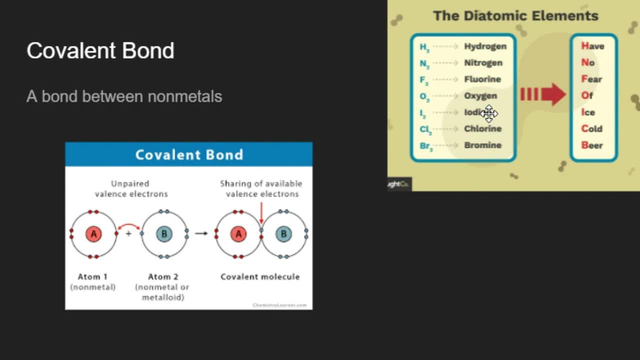 and oxygen being like somewhat high, but fluorine is higher. so what'll happen? the result is that the fluorine would hold the oxygen- i mean the electrons being shared more towards the fluorine, um making the fluorine the mild charged plasma electron or the thread of the blood salamander. 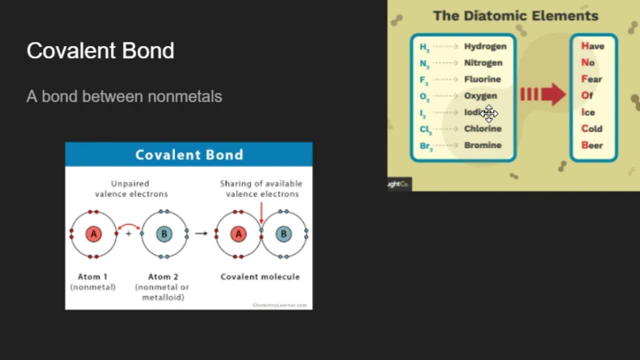 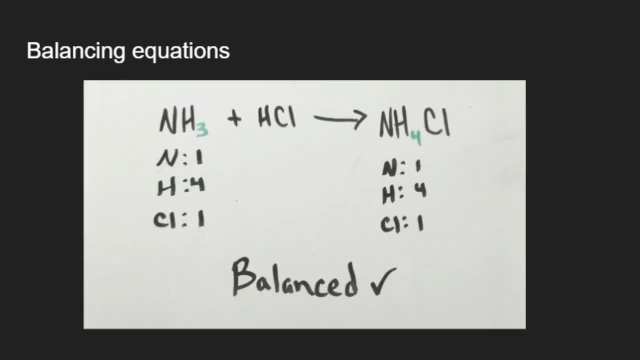 fluorine more slightly negatively charged, while the oxygen being slightly positively charged, okay. so, um, yeah, this is something you should also get used to at a early time, just like balancing equations. um, balancing equations isn't really that difficult. anyone can do it. um, all you need is just basic mathematical skills and just division as well. 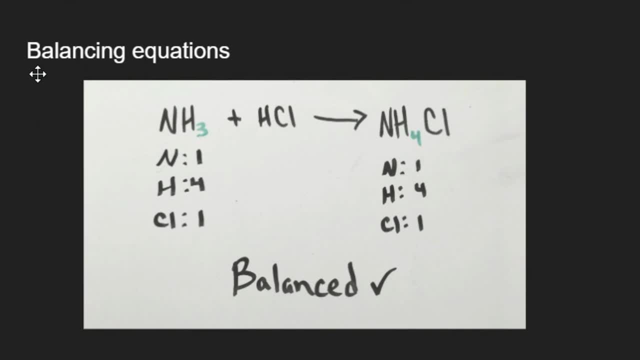 but, um, oh, one of the things that you should know is, whenever, um, they're like odd numbers or something like that, and you get like some decimals or anything, just multiply it and make sure it is a whole number. it shouldn't be a fraction or decimal. okay, it should be a whole number. now, yes, this is a good way to not um, solve like: 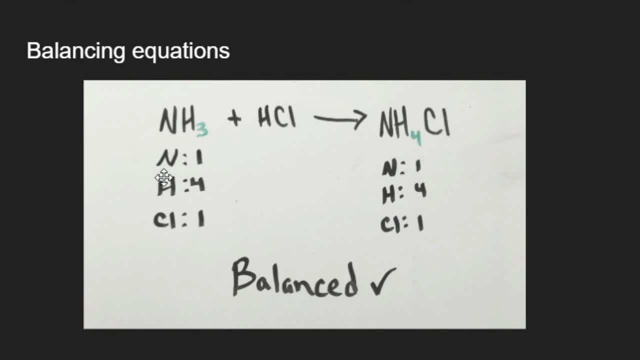 balancing equations, because here you can see he, this person, has listed out how many um, of how many atoms are in this on the left hand side, and, uh, how many there are in the right hand side. and, as you can see, it's balanced. so let's count. 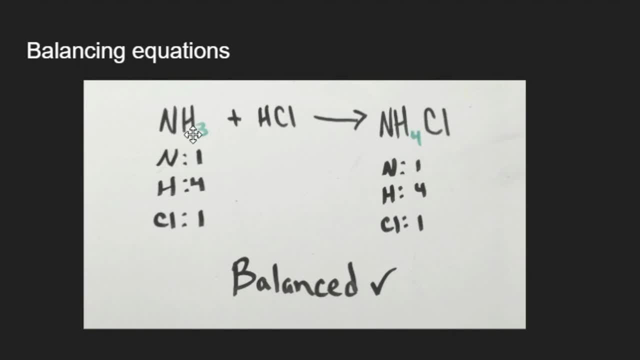 again n, yeah, it has one h, three, there's three h's, uh, hydrogens, and then there's another hydrogen, so okay, that's correct, and there's one chlorine, that's correct, and it's gone. here again there's one h, i mean, um, sorry, one hydrogen, okay, there's four hydrogen, okay, and there's one. 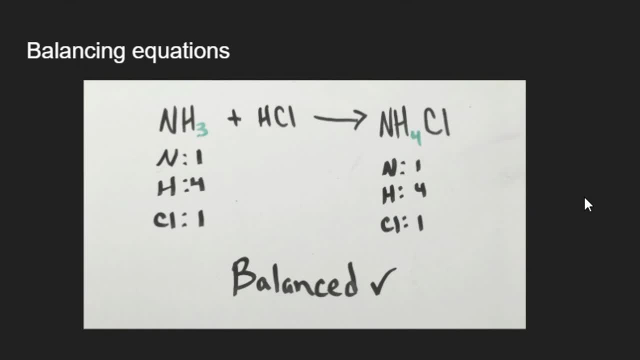 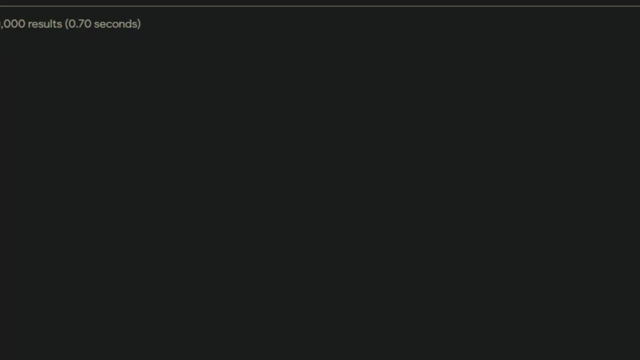 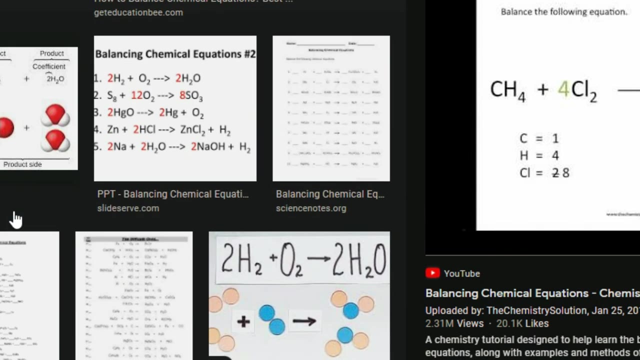 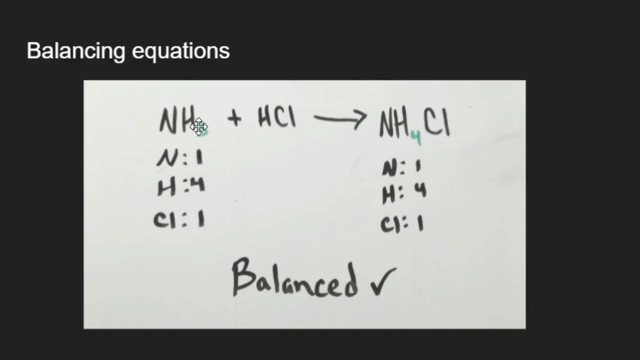 that's it. so, um, wait, let me search for someone, okay, so you have seen that in this example there isn't exactly like a a number in front of like a number like right here or anything, and that's like, if you can this, um, okay, one thing that you. 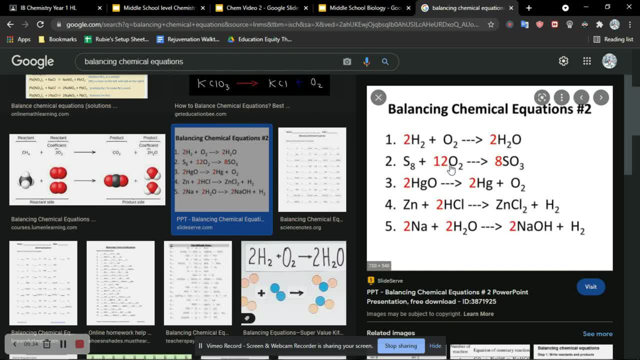 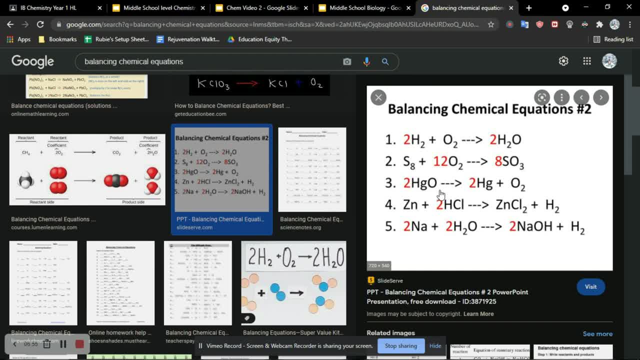 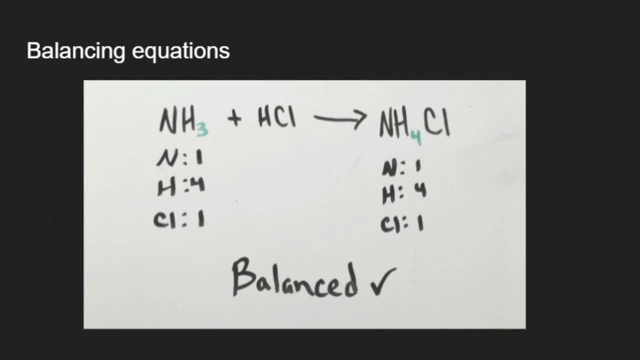 two oxygen, so the two years being multiplied to both of them, it's gonna be hg202. okay, just make sure you remember that. do it confused labs, and i think that's it for today. thank you for listening. um, i'll, i'm not sure if i should make it more difficult, difficult. 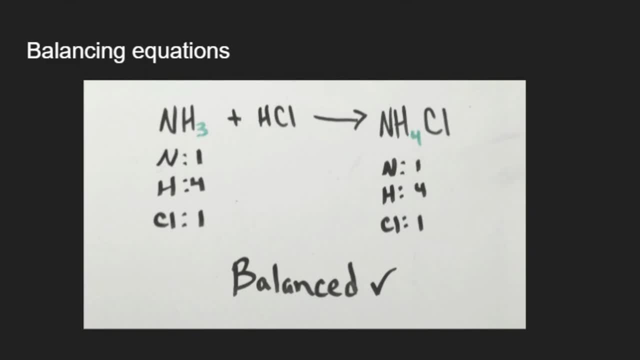 i'm gonna have to probably think about it. maybe i might make it a little harder because, um, it gets really difficult later on. so it's it's better if you guys learn like the complex stuff early or get like a brief, you know- view of it. so yeah, goodbye, have fun. and i'll see you guys in the next video.